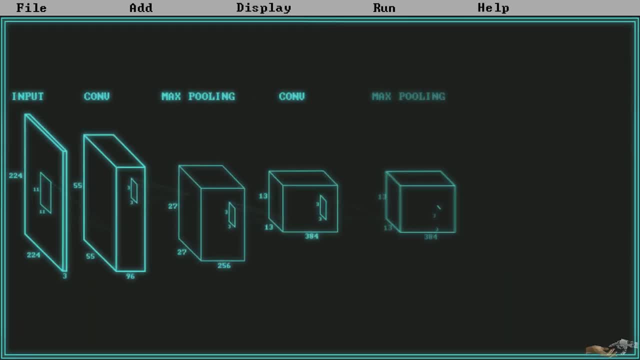 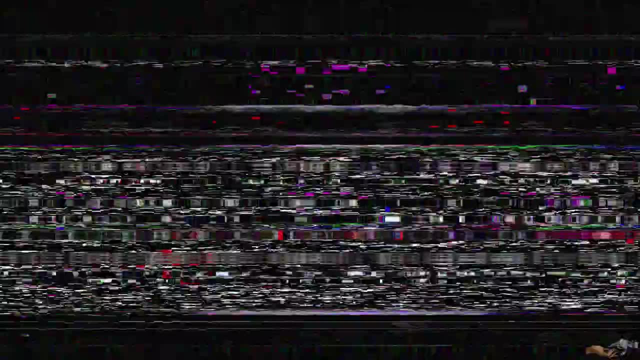 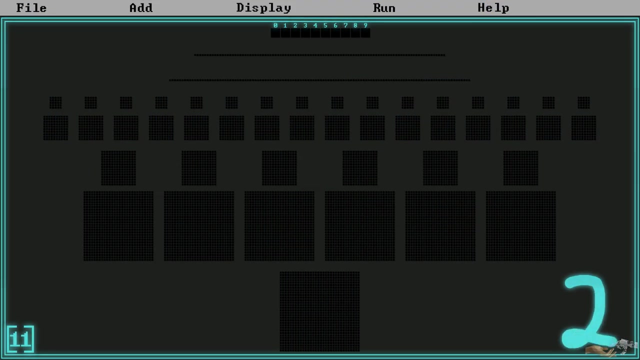 popular and important neural network architecture: the convolutional neural network. For our discussions on convolutional neural networks, we will go with a very common example: number recognition. The reason this example was chosen is because of this great interactive resource by Adam Harley, a robotics PhD at Carnegie Mellon University. I have linked. 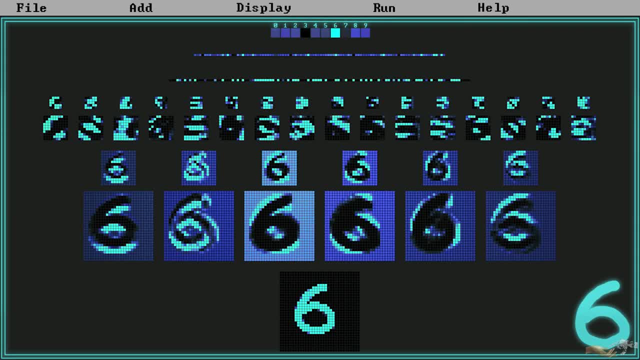 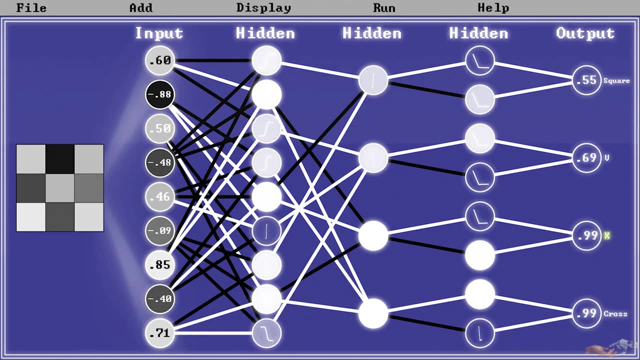 the resource in the description, so that you too can experiment with it and see the internals of a convolutional network. Now, if you can recall from our example on an image pattern recognizer using a feedforward network, we set up an idealized system and made the assumption that each hidden layer in our network would build upon further layers. 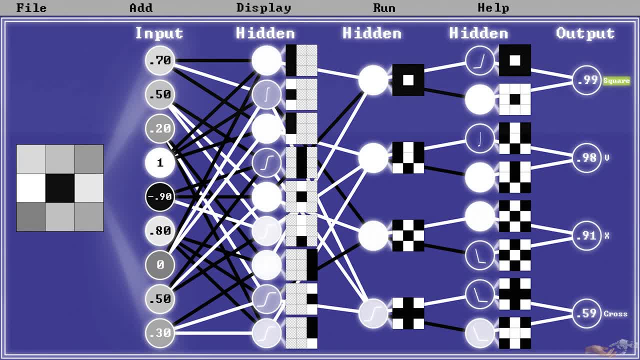 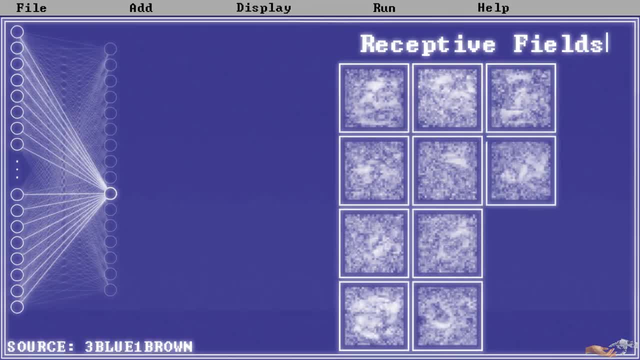 of abstraction from vertical lines to combinations of vertical lines. However, in actuality, as we explained, this wouldn't happen and the receptive fields in the network would be a lot more random to the human eye due to the architecture of feedforward networks. 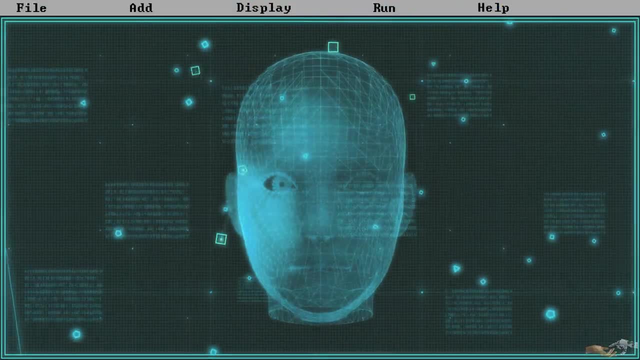 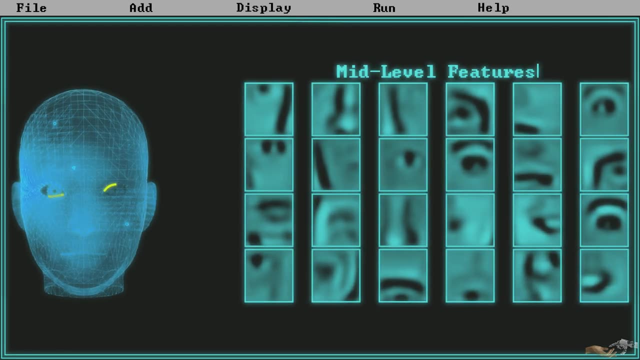 and how they compute With convolutional networks. however, this isn't the case and we could, to some extent, see these layers of abstraction building up. Before we delve into why and how this happens, let's first set up the structure for the network we will be using. As with our previous example, in image recognition, the input will: 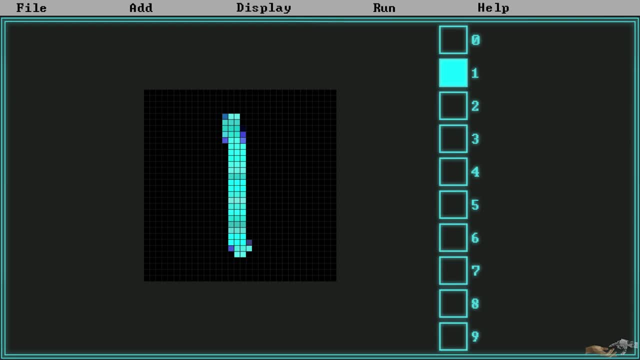 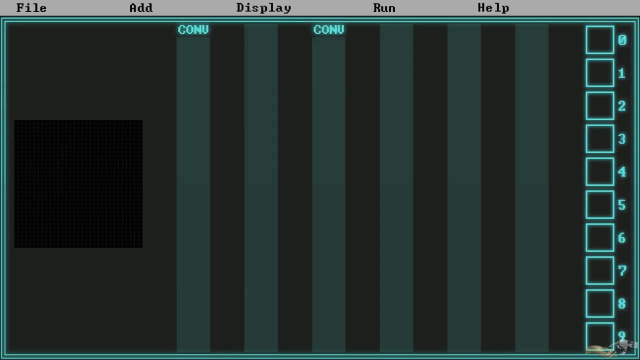 be the individual pixels of our image, and the output, the patterns we are trying to classify. In this example's case, we have 10 outputs, numbers 0 to 9.. For the layers in between, we will have two convolutional layers, two pooling layers and two fully connected layers. 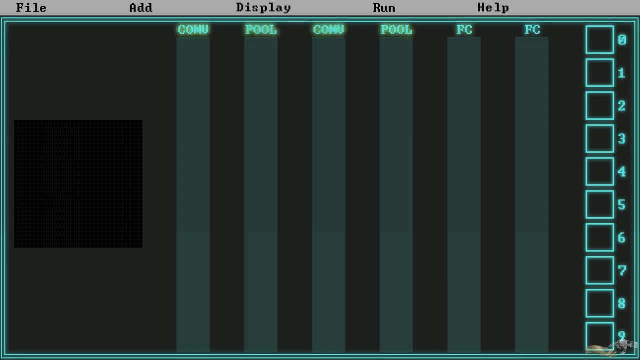 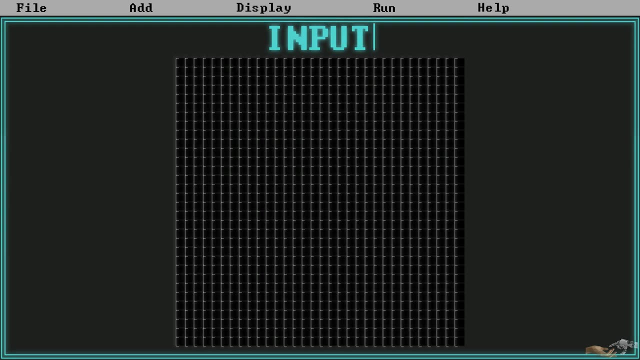 Now, that was a lot of new terminology thrown around, so let's break it down layer by layer, starting with the input. While we have already stated that the input is the individual pixels of the image, I want to mention some important details about how a computer views. 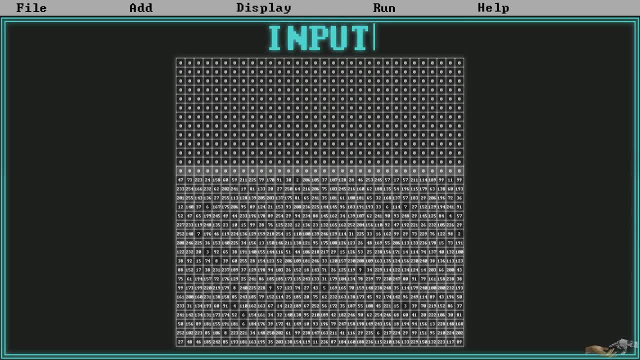 this image. Every image is a layer and each layer is a pixel. The input is a pixel and every image in a digital device is stored as a matrix of pixel values. This is referred to as a channel, a certain component of an image. Now, with a typical digital camera, 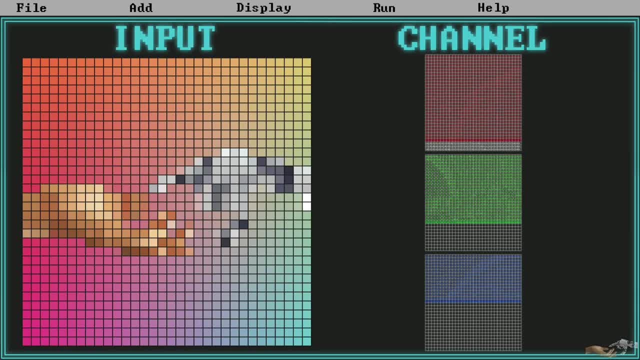 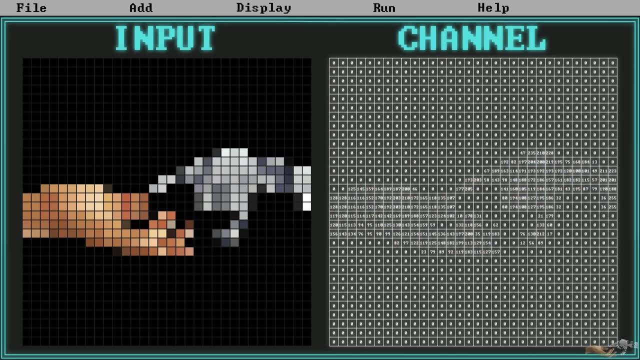 every image will have three channels: red, green and blue RGB, which you can imagine as three 2D matrices stacked upon one another. For the sake of simplicity, we will assume our input has just one channel: the luminance of the image, with the value of each pixel. 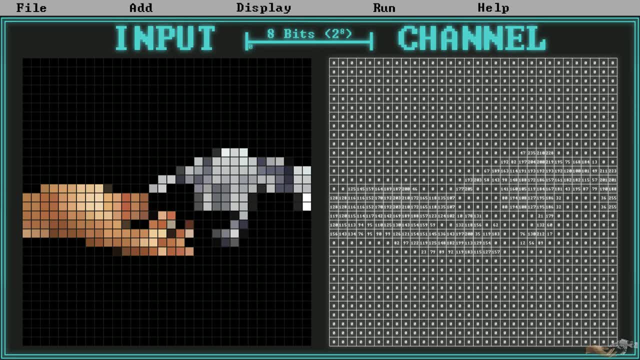 represented in 8 bits. In other words, the pixel values will range from 0 to 255, with 0 indicating dark or transparent luminance and 255 as bright. As a side note, digital systems store all types of sensor data and other information. 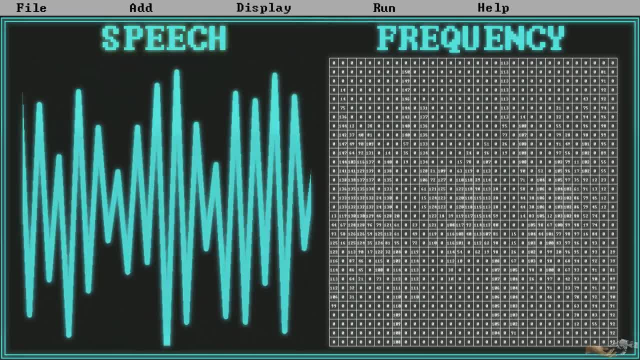 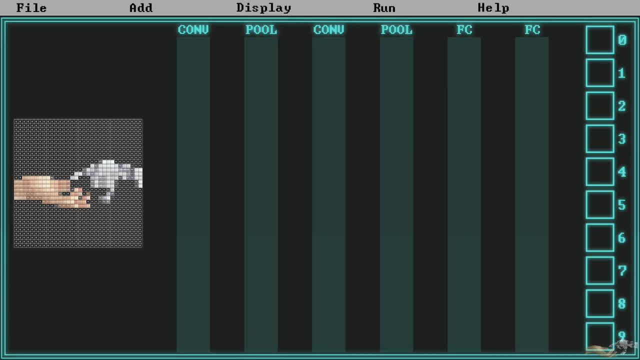 in this fashion, For example, for a convolutional network that would operate on speech, we could represent that speech as a matrix of frequency values. Coming back on topic, now that we understand the format of the input, let's finally delve into where the real magic happens: the convolutional layer. As you can assume, this layer and the 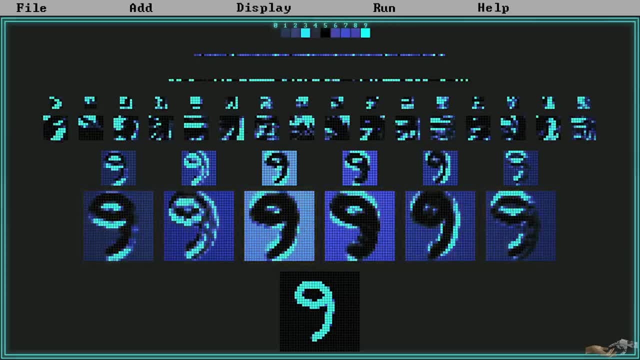 network as a whole get their names from the convolutional operator, which in layman terms, is the mathematical combination, in other words the dot product of two functions to produce a third function. In CNNs this operation is called the convolutional layer and the function is called the dot. 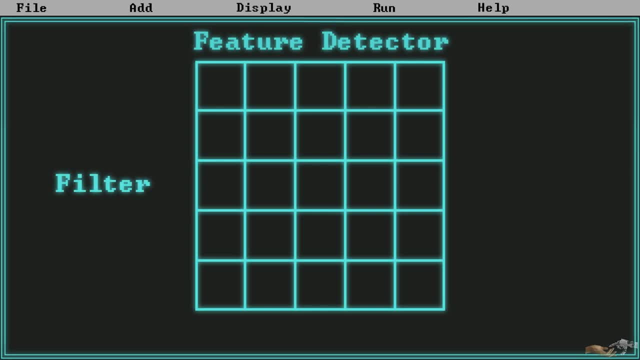 product of two functions. In other words, the dot product of two functions is called the dot product of two functions. This is implemented in what is referred to as a feature detector filter or, most commonly, a kernel. You can think of a kernel as a mini-matrix orders a magnitude smaller than the input. 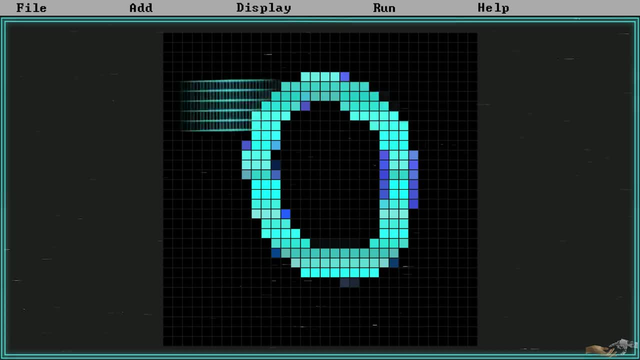 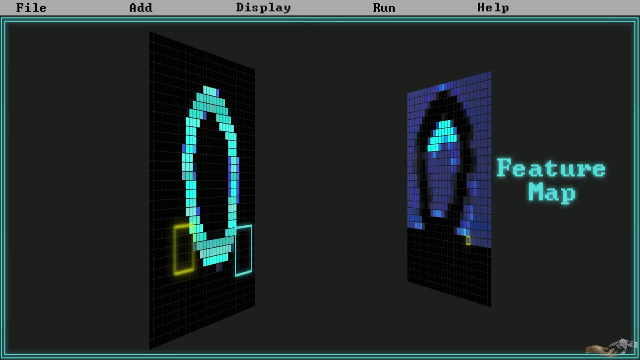 In a convolution operation. then the kernel moves across the input image, taking the dot product of the two matrices and then saving the values to a new matrix dubbed the feature map of the original image. At this point you may be wondering how this is able to detect any features at all. Well, 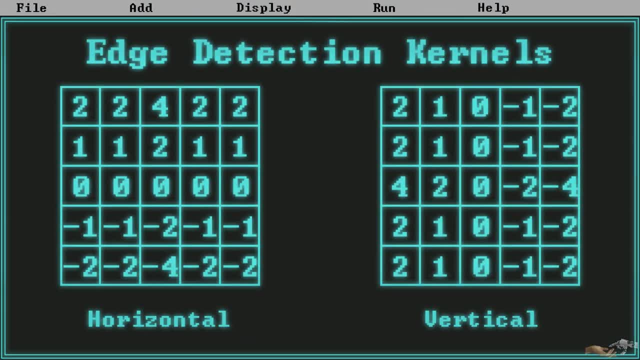 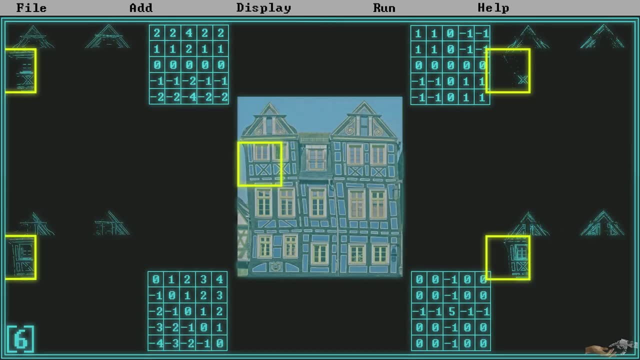 if a kernel is initialized with the values in a specific configuration, they can be used to transform an input image and find various patterns. Like these kernels, for instance, When loaded with the appropriate values and convolved with the input image, produce, is an output which highlights various edges in the photo. 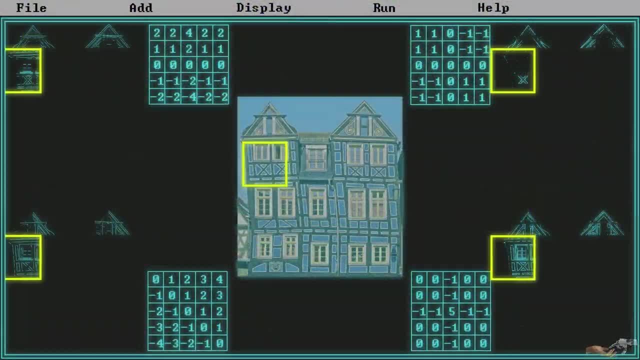 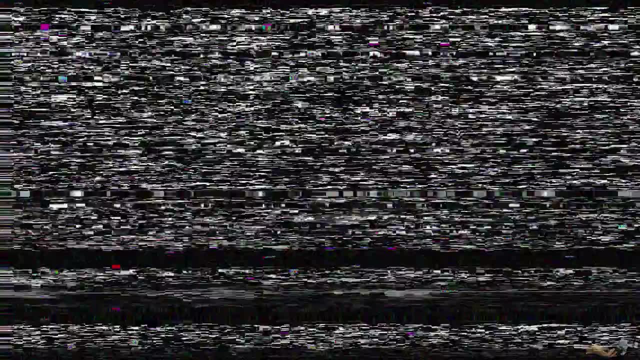 Now I won't delve into the specifics of the various types of kernels in this video, but there are many resources that talk about them extensively, such as Computerphile and their various videos on kernels like the Sobel edge detector. Coming back on topic, as you can see, kernels are essentially ways to do fast computation. 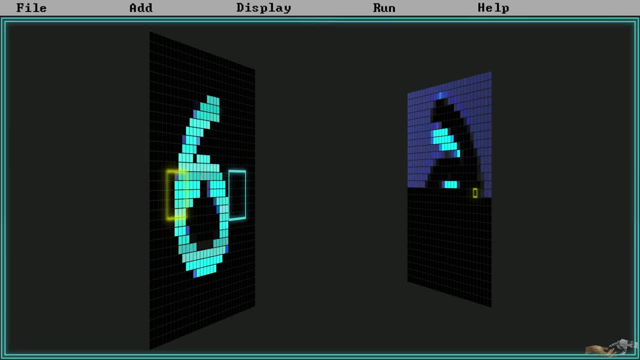 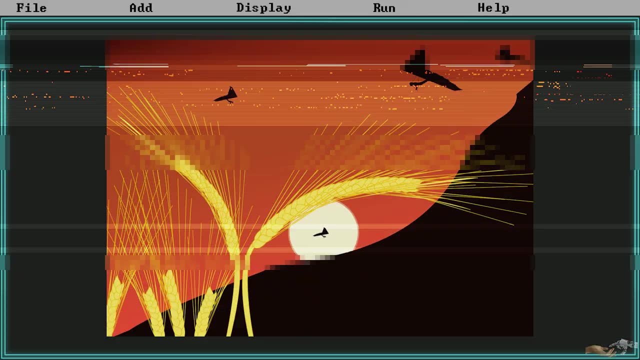 and produce a new output. In this case, we're doing it with an image, with an effect or features highlighted. Programs like Photoshop use these simple kernels for effects like blurs, for instance. Now, when we look at a typical image, take in how much is actually going on. There are. 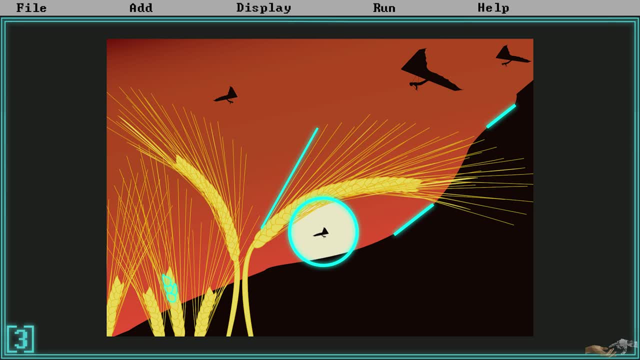 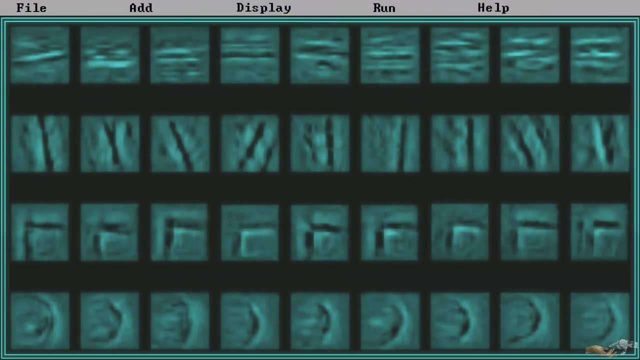 various edges, shapes, textures etc. that stack together to make various objects and the overall image we are looking at At the start of a convolutional network. the types of kernels we'd use would be quite simple and more geometric, detecting things such as edges, corners and simple shapes. 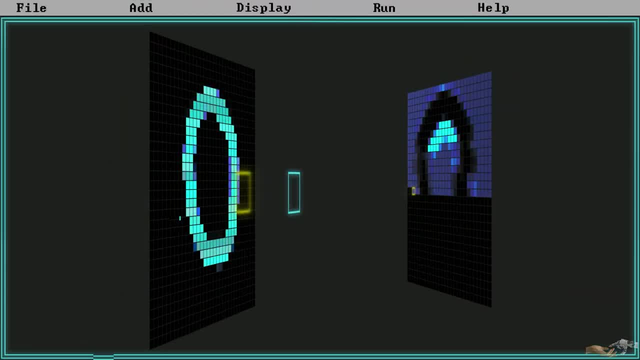 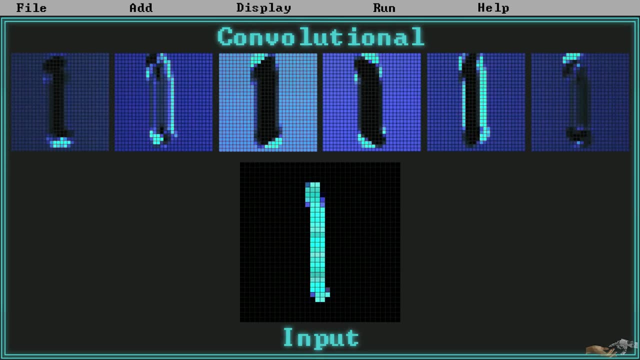 and patterns like a circle, for instance. Additionally, each convolutional layer can have multiple kernels that produce multiple feature maps of their own. So, for our example, we can see that our first layer has 6 kernels, and these kernels are simple patterns like horizontal lines, vertical lines and corners on our drawn numbers. 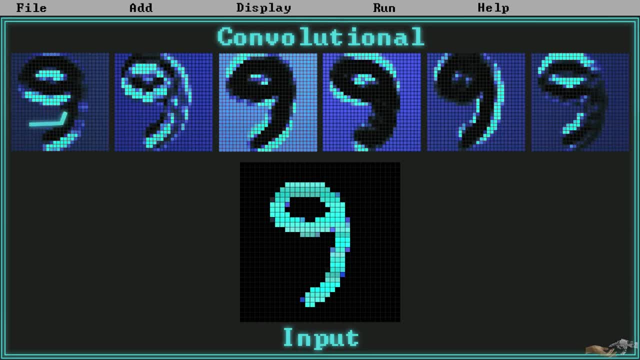 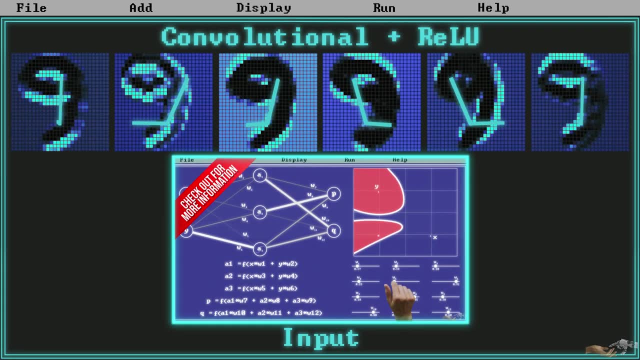 As a side note, for each of the convolved pixels in our feature map, a non-linearity function was also applied, in this instance a ReLU. We discussed this function in previous videos and the need for non-linearity in neural networks, so our feature maps are more adaptable. 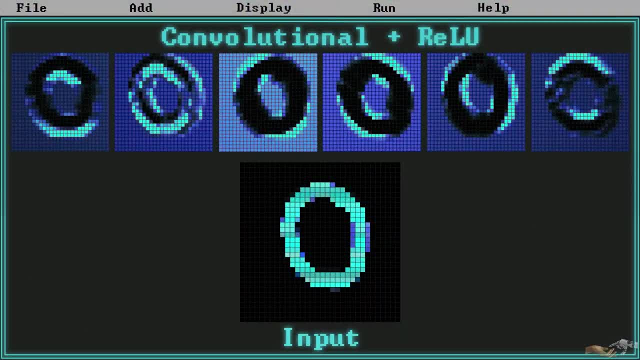 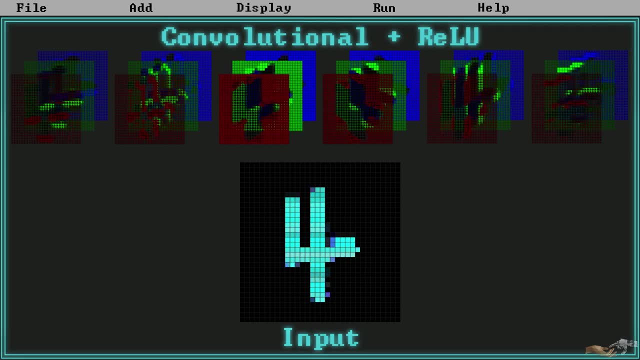 to real-world data. Also, you can now see how complicated this process would become if we had more than one channel, as each channel would have 6 feature maps- in this instance, leading to 18 for an RGB image- and then those feature maps would have to be filtered together or operated a. 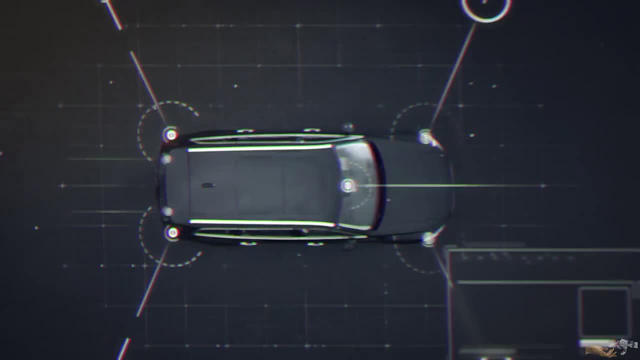 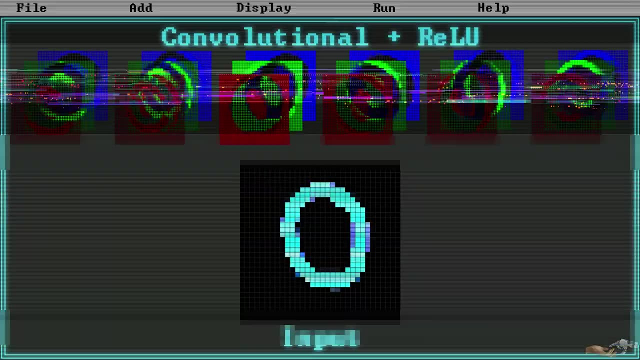 separate way, depending on your specifications. For instance, in a self-driving system, a red hexagon is a stop sign, so we would need separate channels and kernels for those channels. However, coming back to our example, just one channel luminance was more than enough. 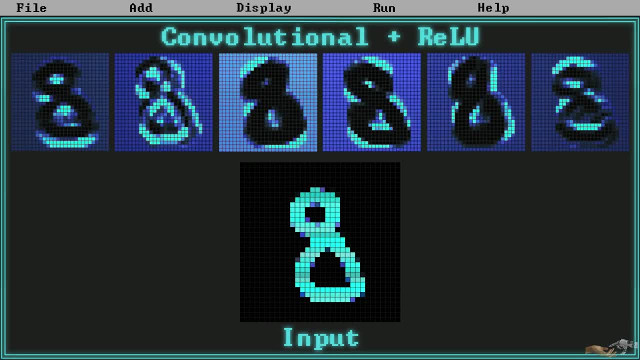 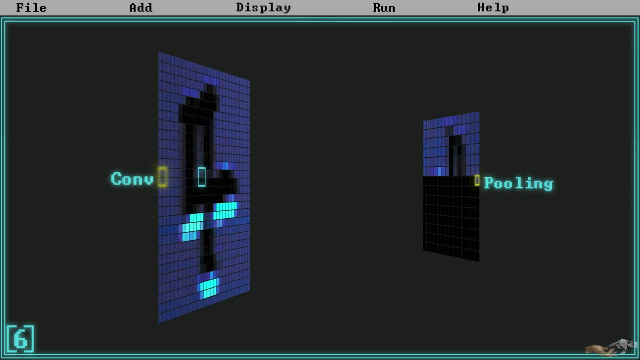 Moving on. now that we have our rectified feature maps, the next layer in CNNs after the convolution is the pooling layer. Pooling layers are used to downsample our feature maps, keeping the most important parts and discarding the rest, and primarily done to 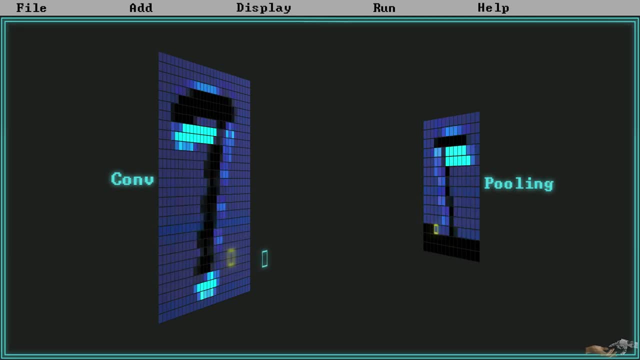 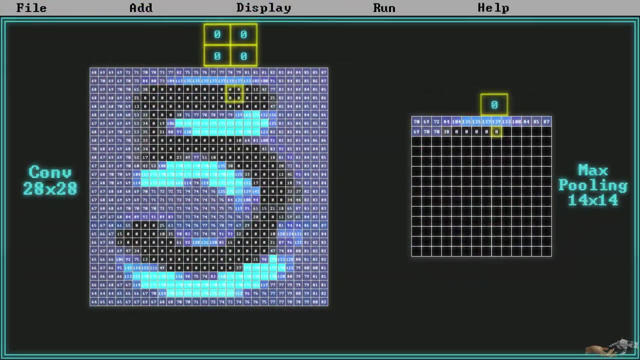 reduce the overfitting rate and so that calculations can be sped up in later layers due to the reduced performance of the image. The type of pooling our network implements is max pooling, in which we take another kernel and slide it across our input feature maps and the largest pixel value in that region. 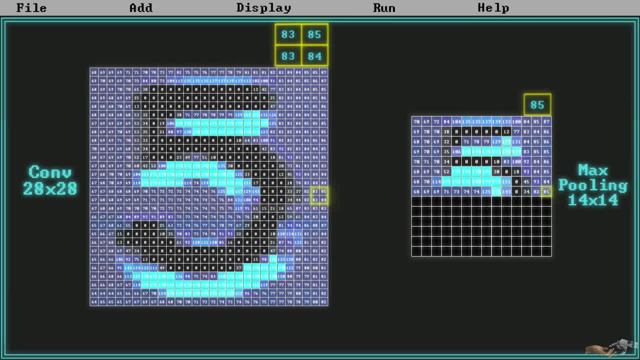 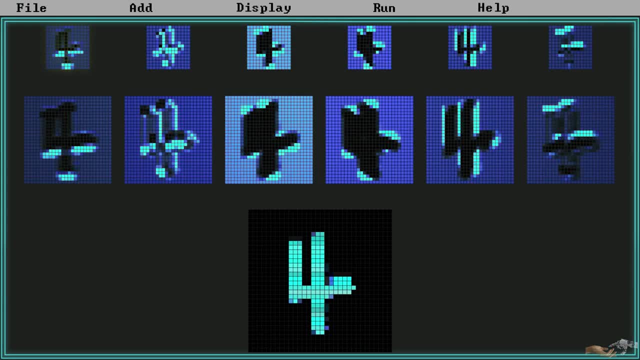 is what is saved to our new output feature map. As you can see, in this number classifier the max pooled layer still retains the important information from the convolutional layer, while being smaller in spatial size, For instance, in this feature map you can still make up. 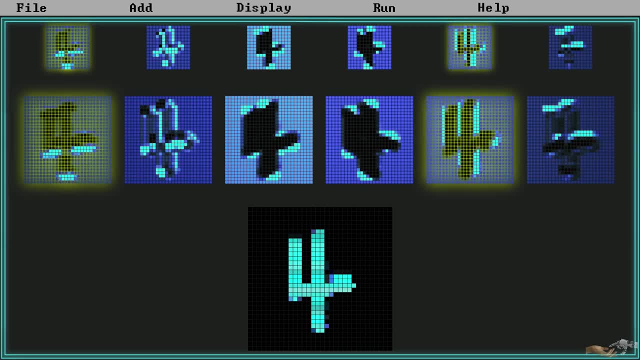 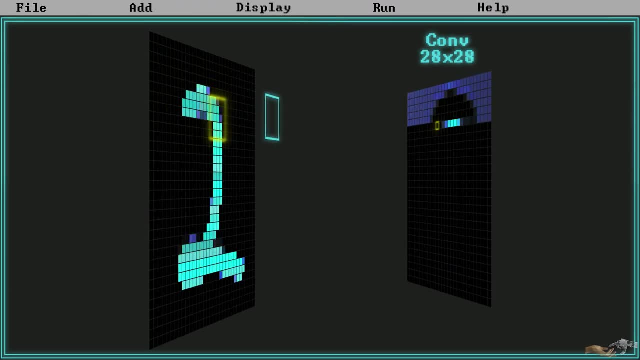 the horizontal lines and in this one the vertical, from their respective original feature maps. So now with the defining layers of the convolutional neural network understood: A, the convolutional layer which extracts features, and then B, the pooling layer which downsamples the feature. 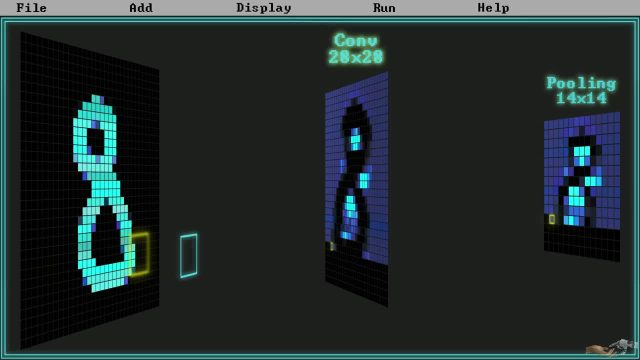 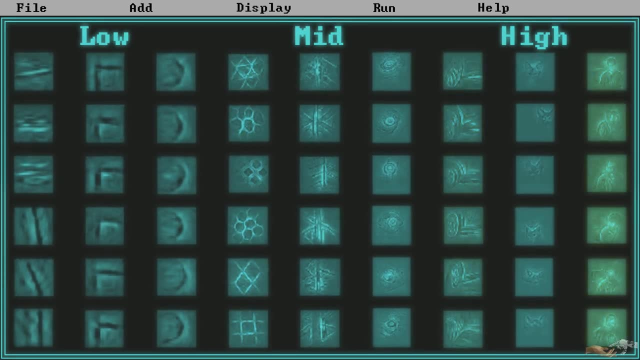 maps. the next step is repeating these layers to build up more abstraction in the network. As stated earlier, in later layers of the network, more complex kernels are incorporated that detect shapes, objects and other complex structures, which is done by leveraging the previously generated feature maps and their detected simple features to build more complex. 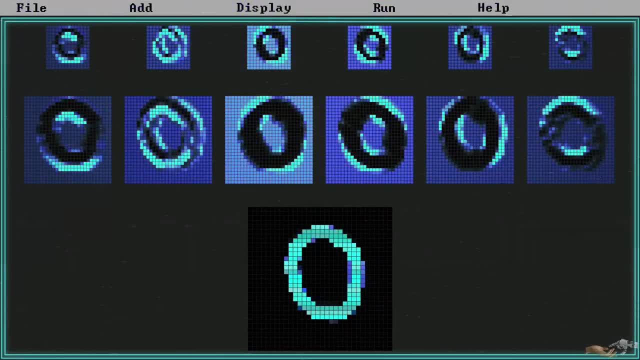 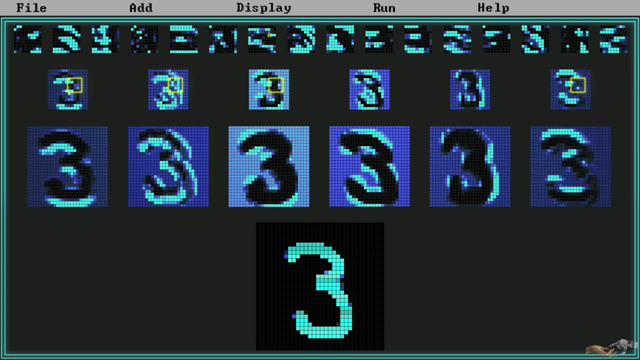 ones. This is essentially the definition of abstraction. You can see in our example that in the next convolutional layer there are 16 kernels, and these kernels are now much more complex. In the first convolutional layer we were detecting simple edges and corners, and now, as you can, 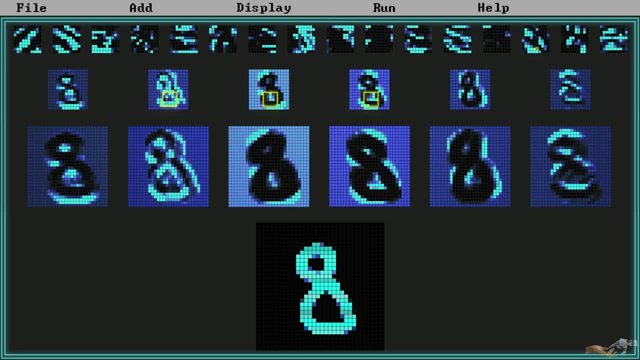 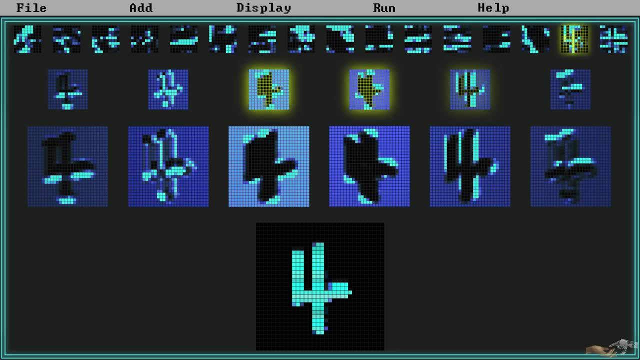 see, horizontal and vertical edges are being combined, as well as other simple shapes from the previous feature maps, For instance, with this drawn 4. you can see this feature map combining both horizontal and vertical edges from various earlier layer feature maps and resembling a bit of the structure of a 4, or with these feature maps of a 5, where diagonal 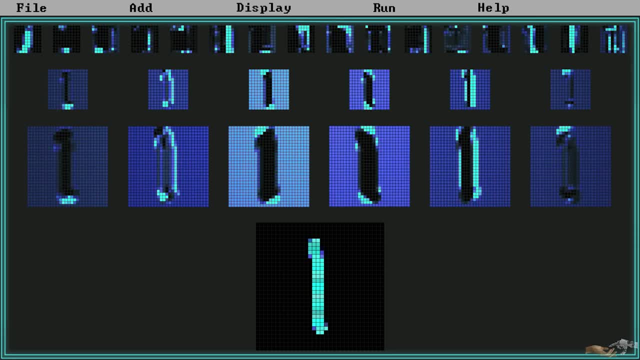 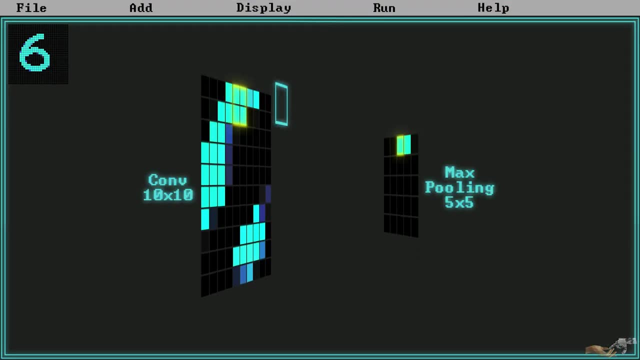 lines and S-shaped patterns are being detected. As you can see, similar higher level features are present for all numbers. Now, after this convolutional layer, just as before, there is no need to apply the feature maps on the actual numbers to reduce the spatial dimensions. 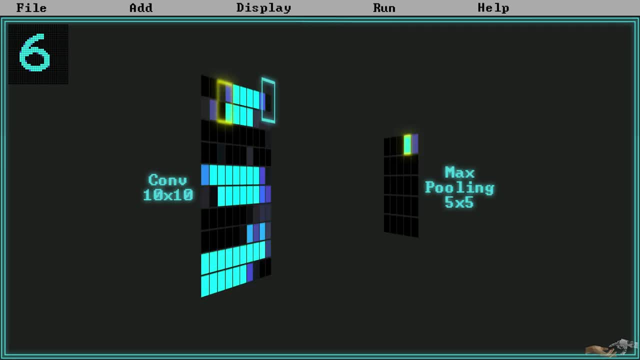 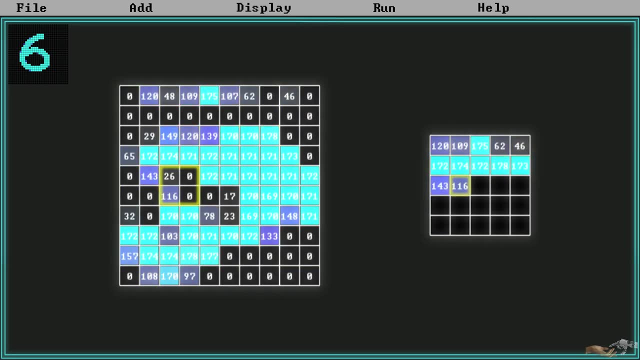 of the feature maps before the fully connected layers, As seen here. with these newly pooled maps they look a lot more random to the human eye, since the spatial resolution is not very low. however, to a computer, they are just the key points in a matrix that represent a drawn 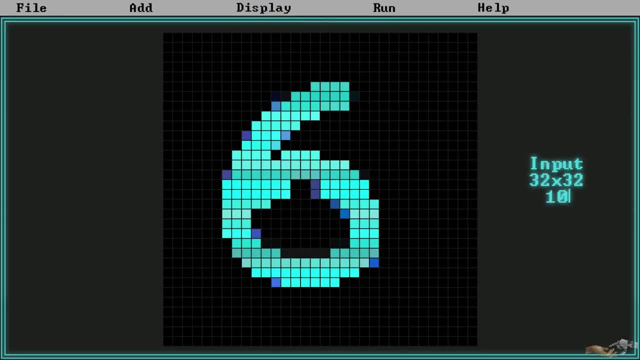 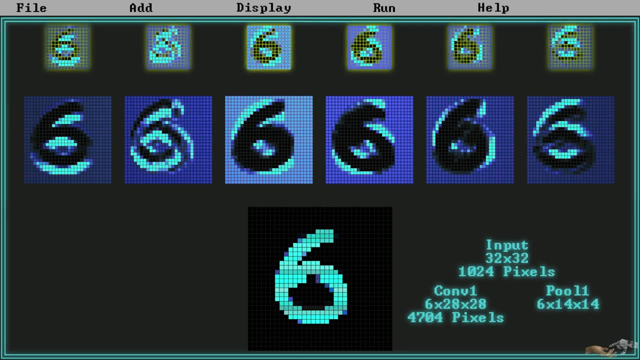 number. You can also see now why we needed these pooling layers: From a raw input 32x32 pixel image with 1024 pixels and no discernible features, to 6 low level feature maps of size 14x14 pixels, resulting in 1176 pixels. 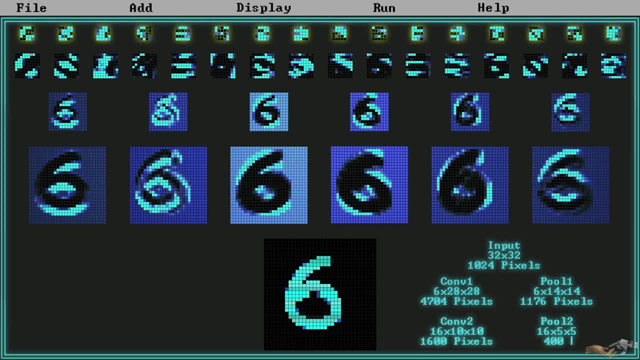 16 high-level feature maps of 5x5 pixels, resulting in 400 pixels, and this, in general, was the whole point of these convolutional and pooling layers: to detect high-level features with as low as possible spatial resolution, and why this part of the convolutional neural network is referred to. 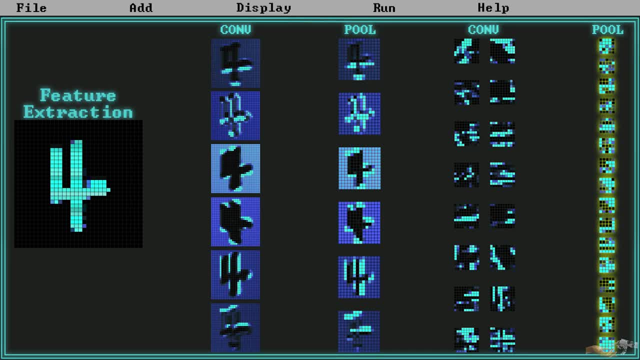 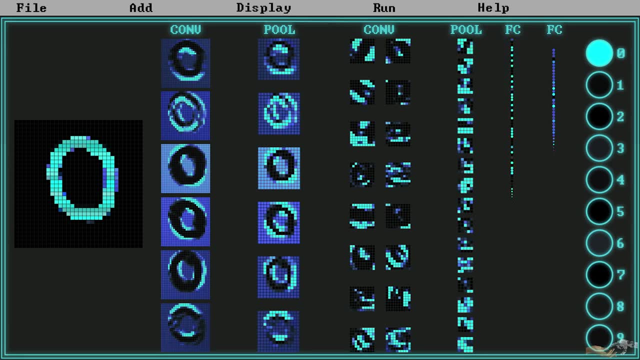 as feature extraction. At this point, with the features extracted, we still need to be able to classify them. hence the second part of a convolutional network: the classifier. This part is comprised of fully connected layers similar to a feed-forward network, except now. 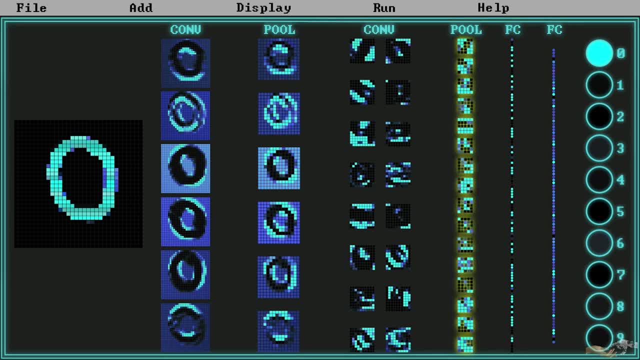 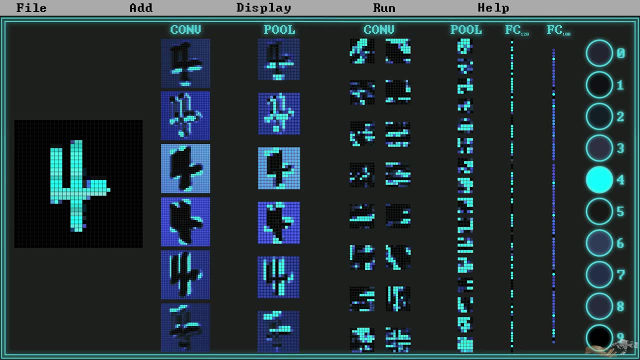 our input to these perceptron layers are the high-level abstracted features from our input rather than the raw input pixels. In this example's case, there are 120 neurons in the first fully connected layer and 100 in the second and, as you can see, these are sufficient. 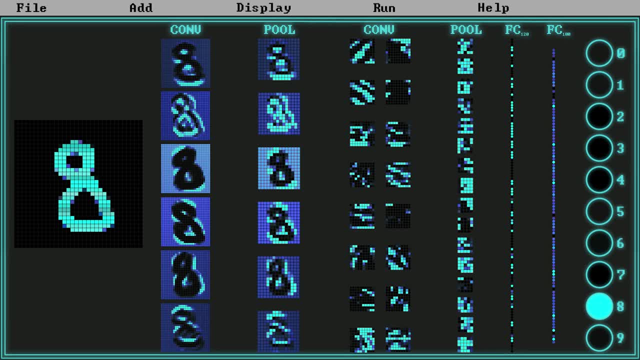 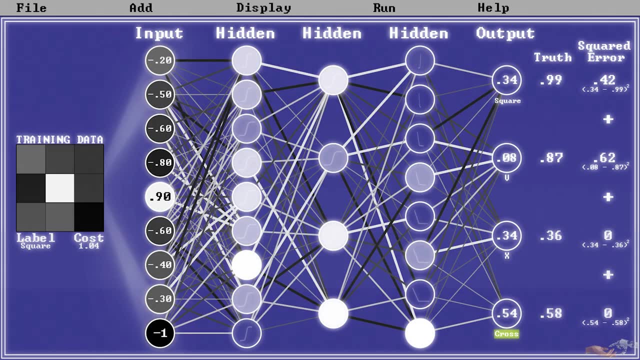 to correctly classify numbers with a high degree of accuracy. Now I hope you can recall, as we've covered in videos past, during the process of backpropagation and gradient descent, the weight and bias values are tuned as the network learns. In terms of convolutional networks, those values 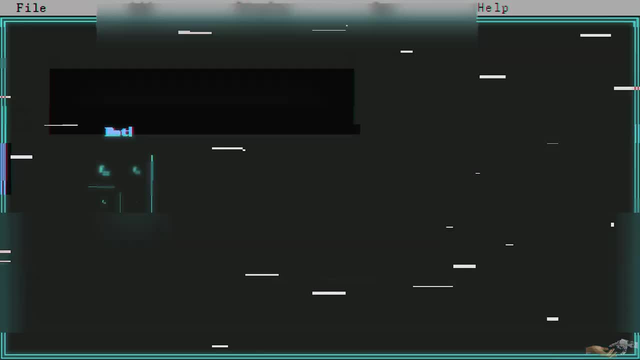 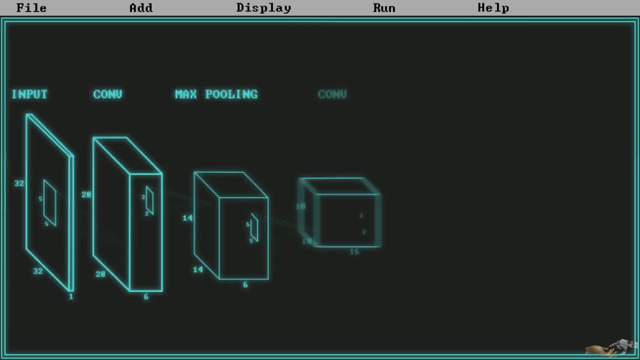 would still be altered during this process, and also other values, such as the kernel coefficients of our convolution and pooling layers, would still be altered during this process. Now, before continuing, I want to stop and highlight the fact that in our discussion of convolutional networks, we have made many generalizations and overlooked many details. 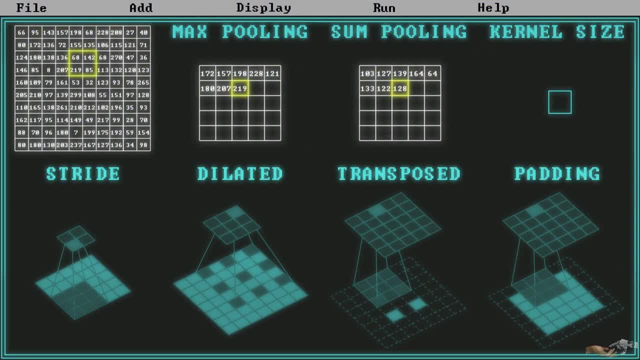 For instance, hyperparameters like kernel size, stride and dilation rate, transposed convolutions and padding, different types of pooling layers, as well as other parameters and hyperparameters in our future extracting layers and their effects on the output, Not to mention the impact of all 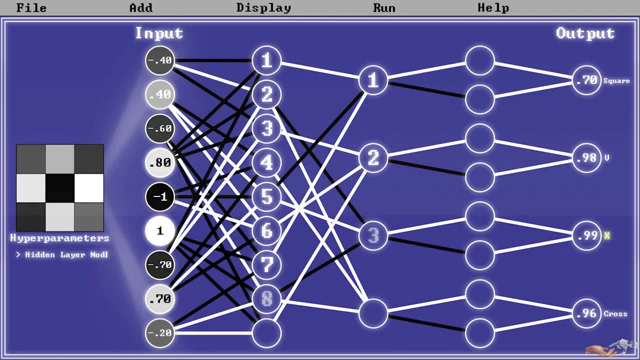 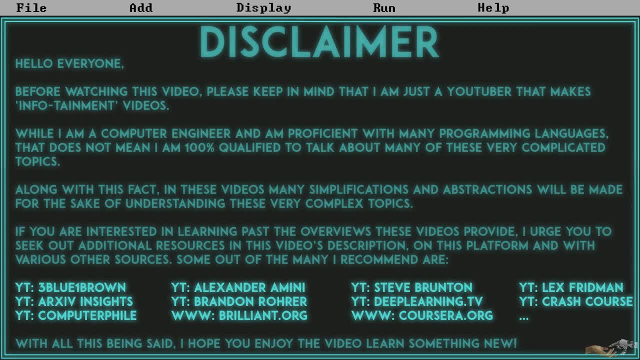 the parameters in our fully connected layers, which we already mentioned in previous videos. If you want more information on these topics, check out the sources in the disclaimer and description below. Coming back on topic, throughout this video we've now seen how and why. convolutional networks.